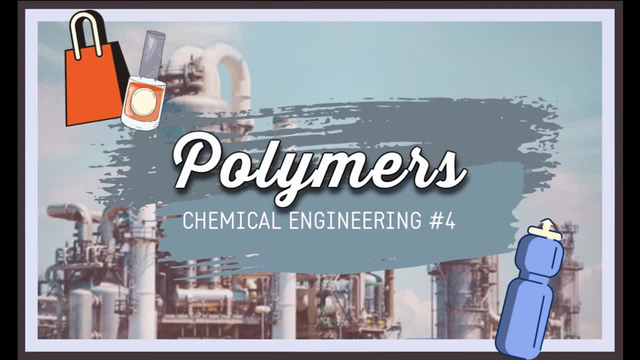 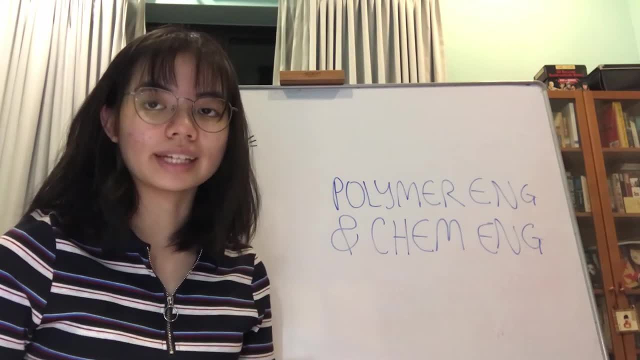 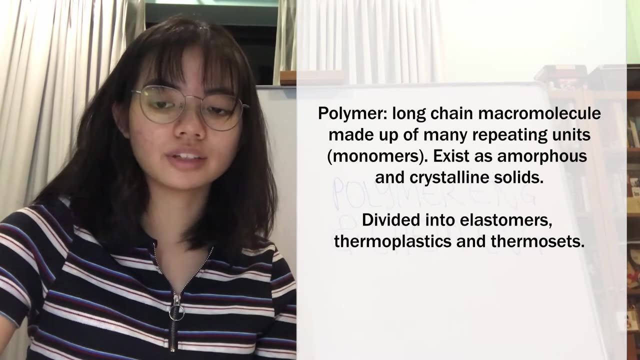 Hi, in our final chemical engineering video, I'll be talking about polymers, polymer engineering and chemical engineering. A polymer is a long-chain macromolecule that is made up of many repeating units called monomers. Polymers exist as amorphous and crystalline solids. Amorphous solids have 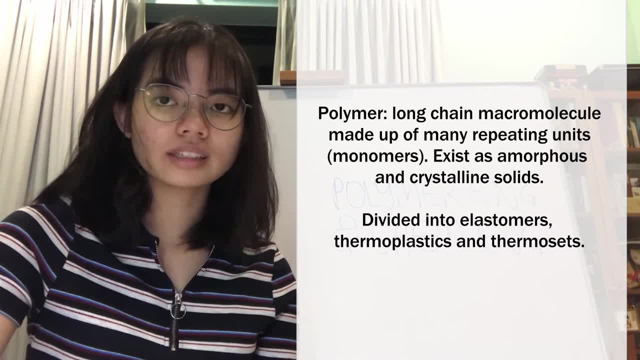 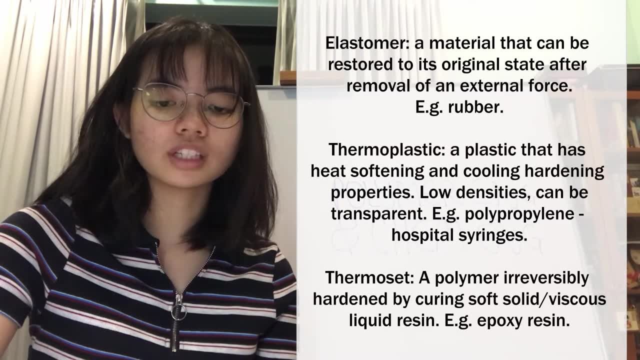 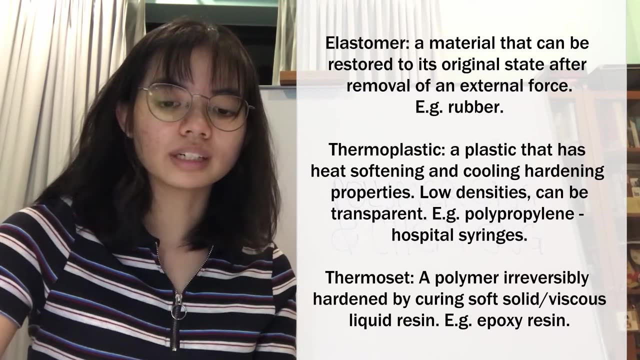 low melting points and are easily deformed, whereas crystalline solids have high melting points, rigidity, tensile, strength and opacity. We can divide polymers into three basic groups: elastomers, thermoplastics and thermosets. So firstly, an elastomer generally refers to a 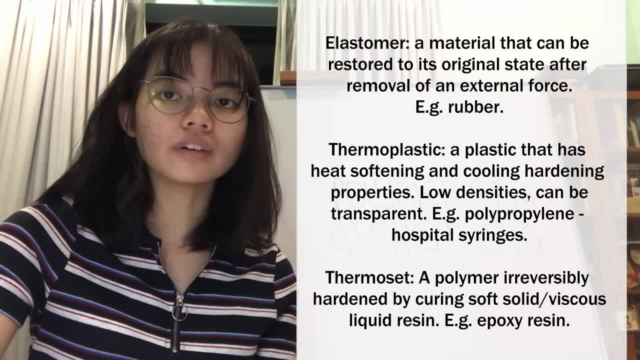 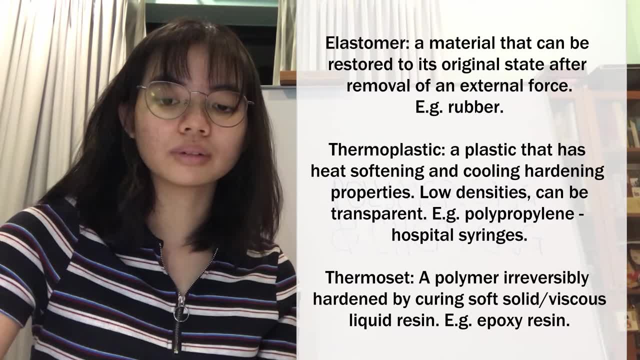 material that can be restored to its original state after removal of an external force. The elastomer is only deformed under weak stress, and the stress can be quickly restored to a polymer material close to the original state and size. An example of an elastomer is rubber. 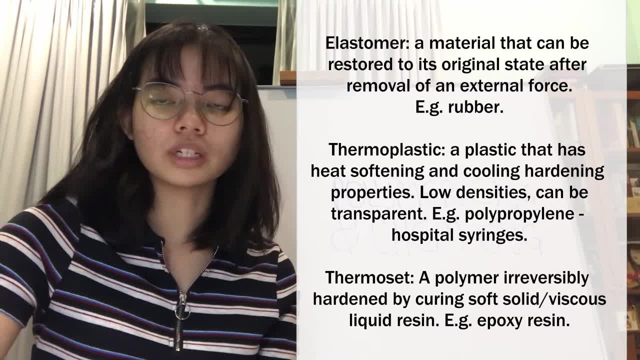 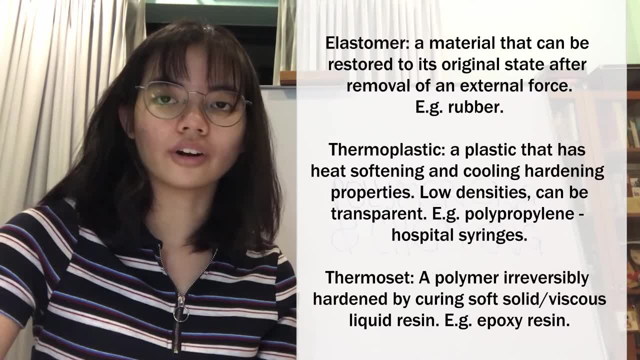 whether it be natural rubber, nitrile rubber, neoprene and more. Secondly, thermoplastic refers to a plastic that has heat-softening and cooling-hardening properties. Most of the plastics we use in our daily lives fall into this category. The plastic becomes soft. 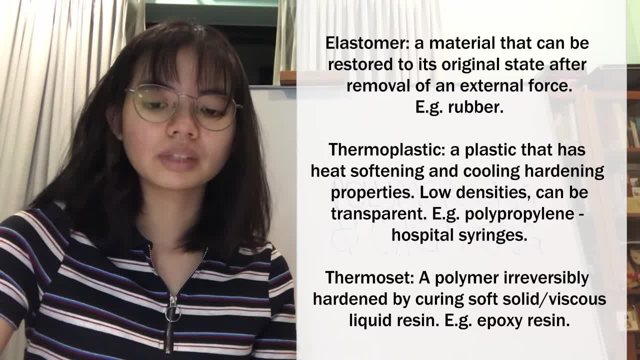 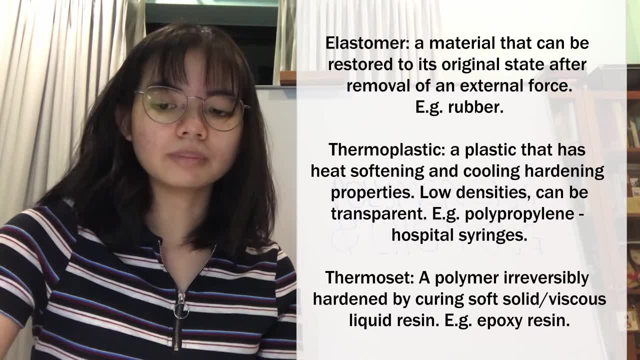 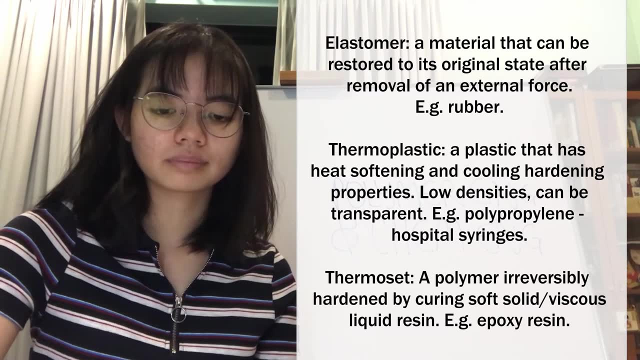 and even flows, when heated and upon cooling becomes hard. This process is reversible and can be repeated. Thermoplastics have lower densities and properties such as transparency, which make them ideal for consumer products and medical products. They include polyethylene and polypropylene. Finally, a thermosetting polymer or a thermoset. 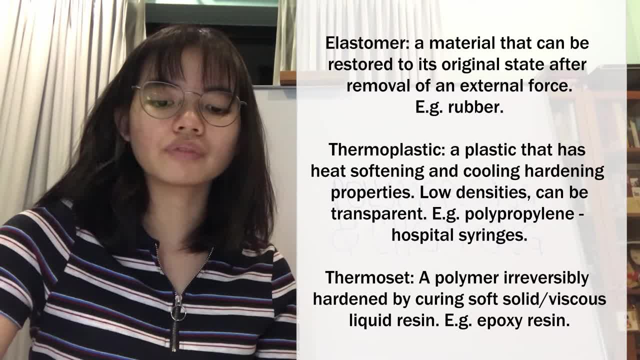 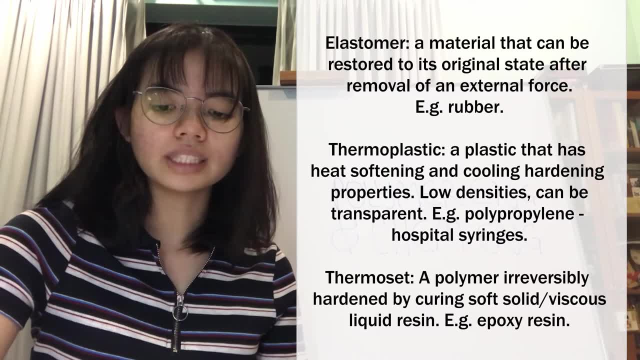 is a polymer that is irreversibly hardened by curing from a soft, solid or viscous liquid, prepolymer or resin, forming a product by a cross-linking curing process in combination with various necessary additives. It is liquid in the early stage of the manufacturing or molding. 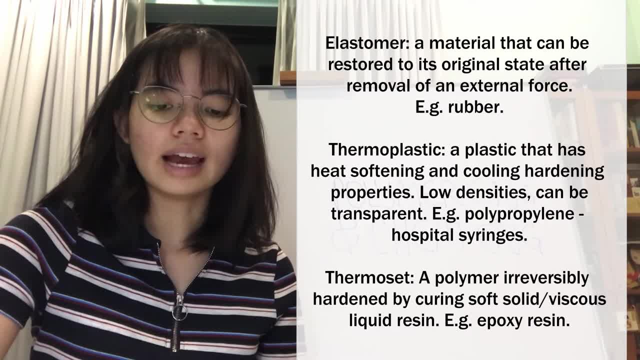 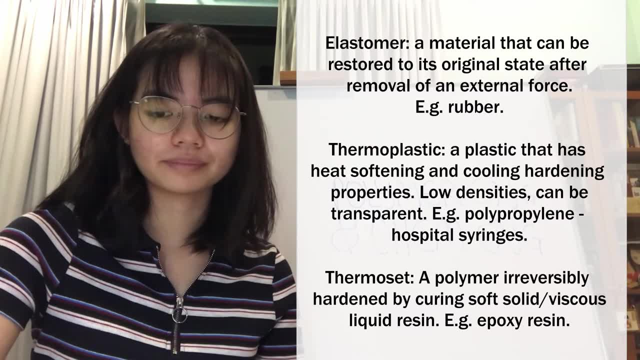 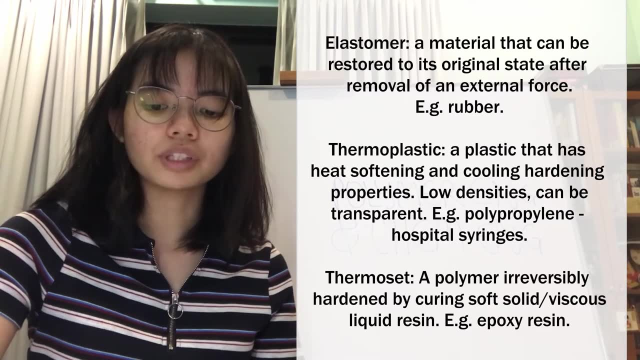 process and it is insoluble and infusible after curing and it cannot be melted or softened again. An example of a thermoset is polyesters and epoxy resins. When we chemically synthesize polymers through addition or condensation polymerization with 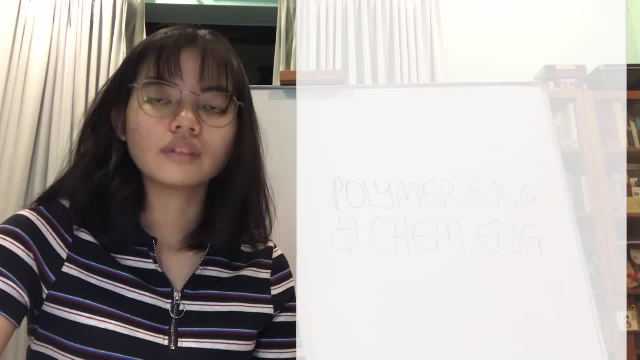 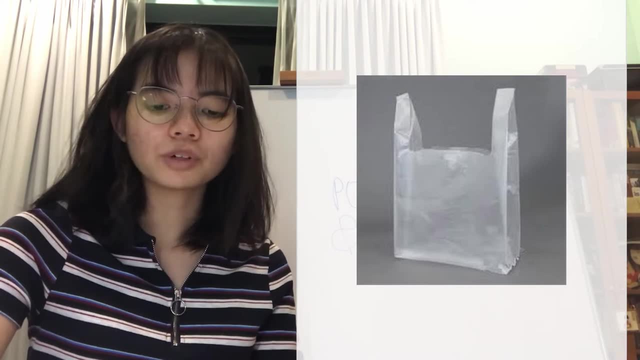 these properties in mind, polymers can turn out to be very useful. For example, polyethylene, a polymer of ethylene, is widely used for making plastic bags and bottles. Polypropene is used for making crates and ropes, while polychloroethene and polyvinyl chloride or 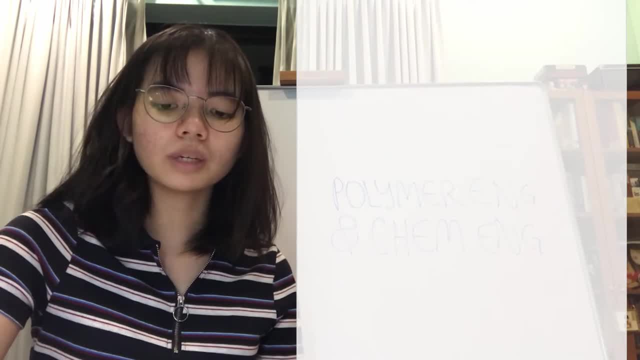 PVC are used for making plastic bags and bottles. Polypropylene is used for making plastic bags and bottles. Polypropylene is used for making crates and ropes, while polychloroethene are used for making water pipes. Polypropylene, a crystalline and thermoplastic polymer, is 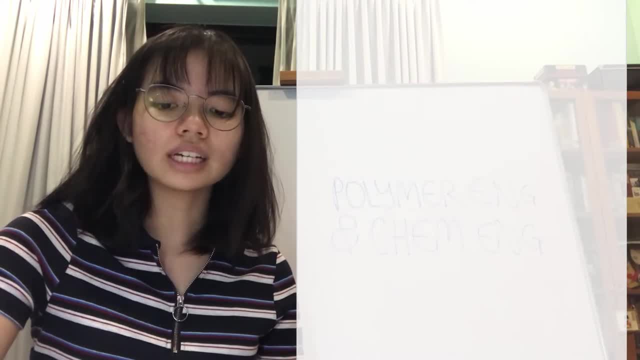 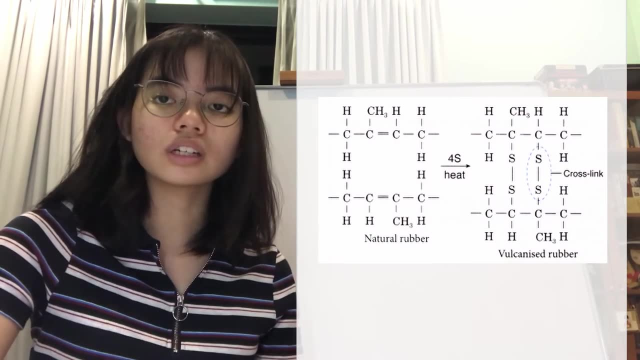 used in the textile industry for making molded objects. Vulcanized rubber is a synthetic form of rubber in which natural rubber is treated with a vulcanizing agent, normally sulfur, to increase cross-lining and cross-linkage in the natural polymer Vulcanized rubber. 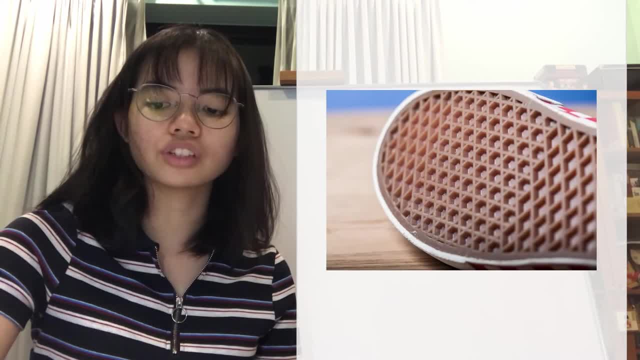 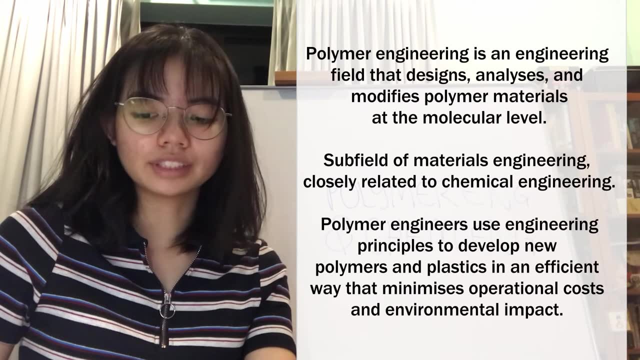 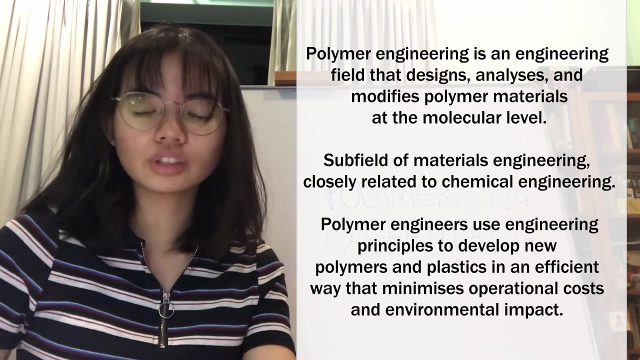 has more strength and resilience than natural rubber and is used to make shoe soles, toys, hockey balls and more. Polymer engineering is an engineering field that designs, analyzes and modifies polymer materials. It is a sub-field of materials engineering and is closely related to chemical. 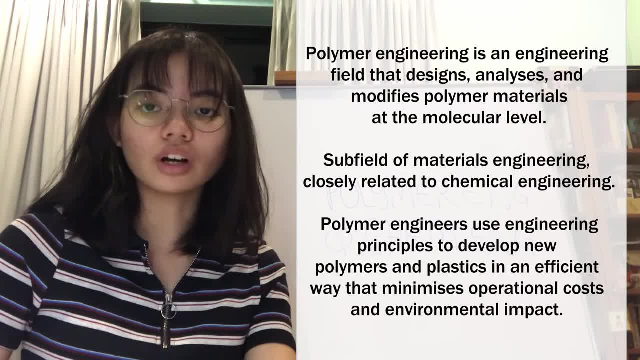 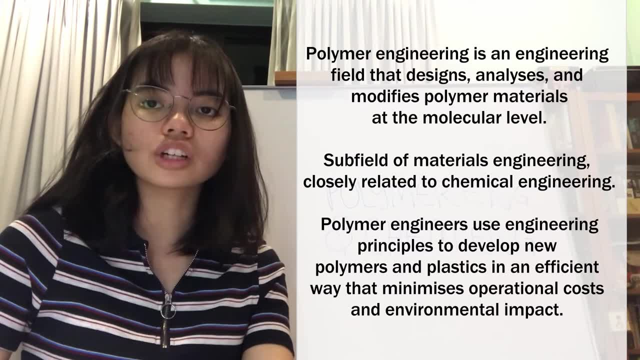 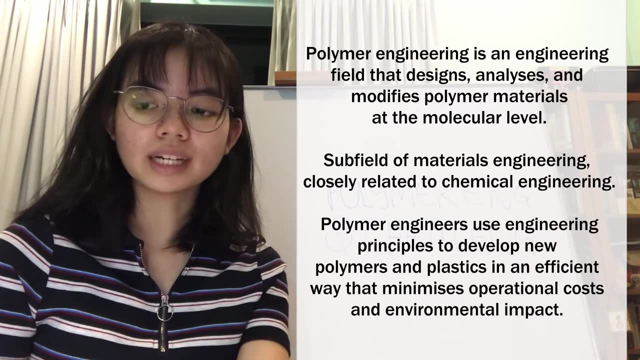 engineering, since both polymer and chemical engineering require knowledge of chemical reactions and interactions between chemical units in order to translate polymers, or any other chemical product, to consumable and marketable quantity to be mass-produced. Polymer engineers, like chemical engineers, use principles of plot design, process design. 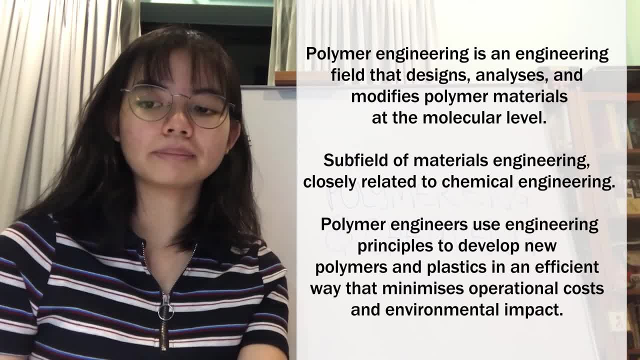 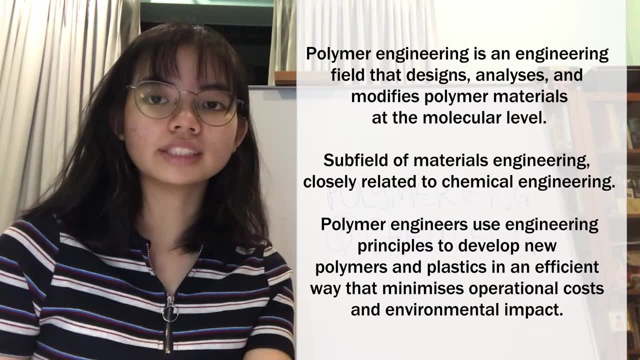 aerodynamics and transport phenomena to develop new polymers and plastics in an efficient way that minimizes operational costs and environmental impact. Polymer engineers study plastics and other polymers at the molecular level, select polymers for new applications and test plastics for new products. They can also work as an engineering. 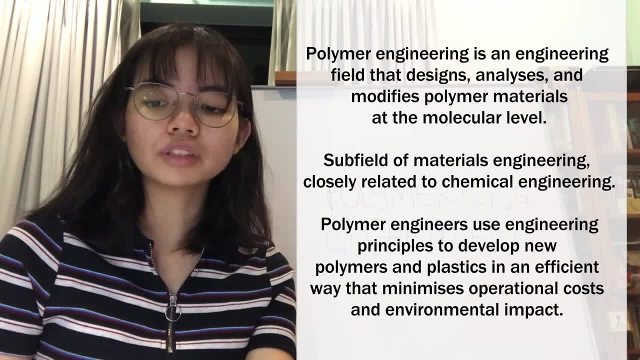 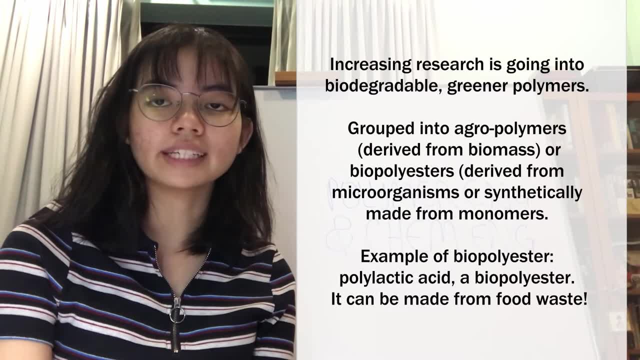 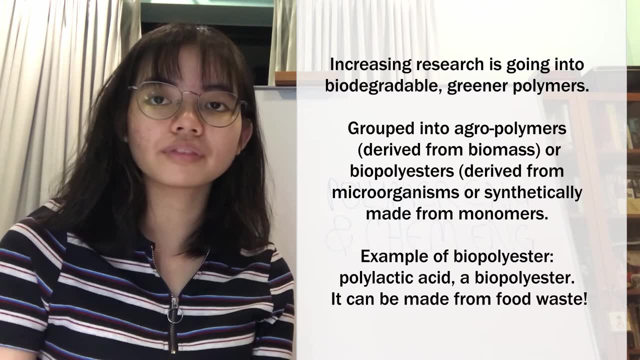 technician or technologist breaking down wood, cotton, petrochemicals and other raw materials to create polymers in an industrial plant: Polymer engineering. Many polymers, such as polyethylene, are non-biodegradable. Increasing research is going into producing biodegradable, greener polymers, which are better for the environment. 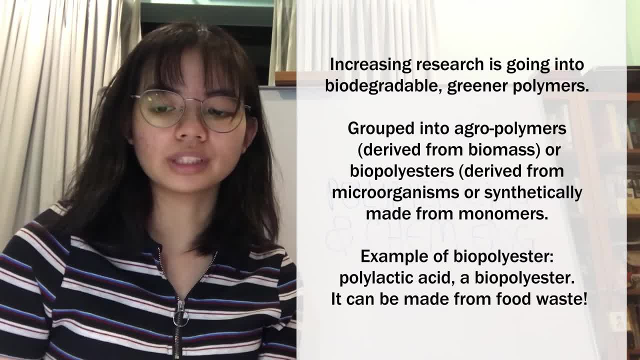 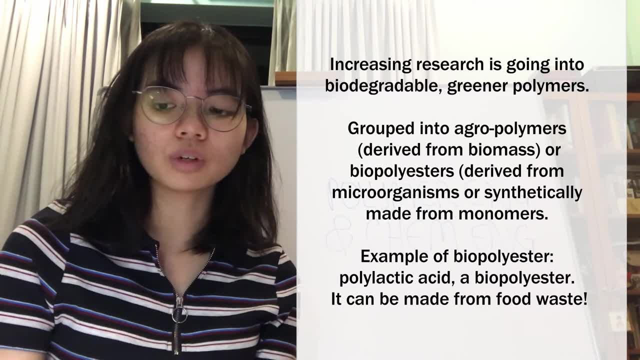 Biodegradable polymers tend to consist of ester, amide or ether bonds. In general, biodegradable polymers can be grouped into two large groups based on their structure and synthesis. One of these groups is agropolymers, or those derived from biomass, and another 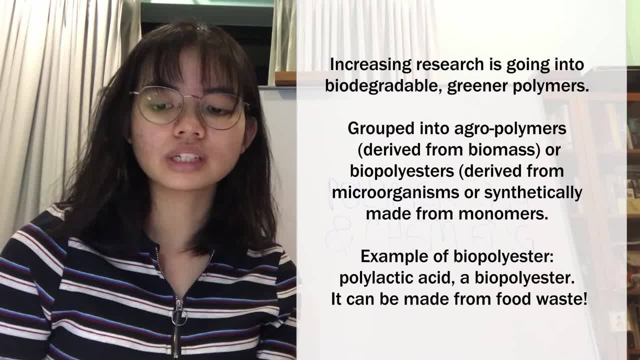 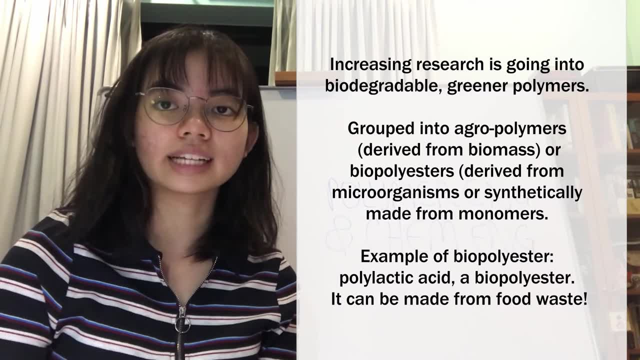 group is biopolyesters, which are those derived from microorganisms or synthetically made from either natural or synthetic monomers- Polylactic acid. An example of a synthetic biodegradable polymer is polylactic acid, a biopolyester In 2010,. 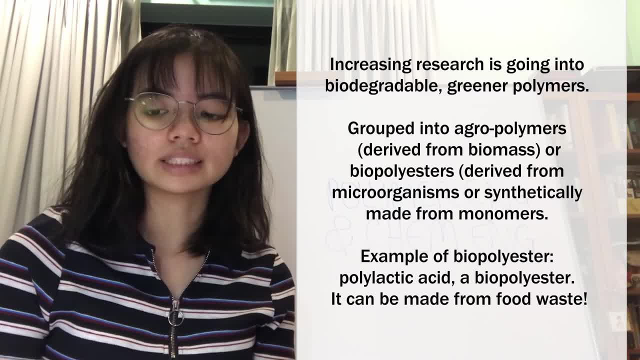 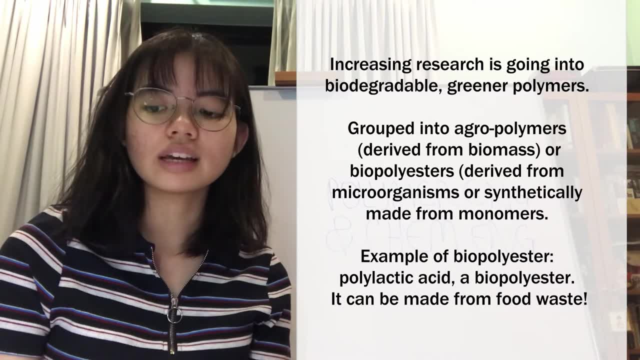 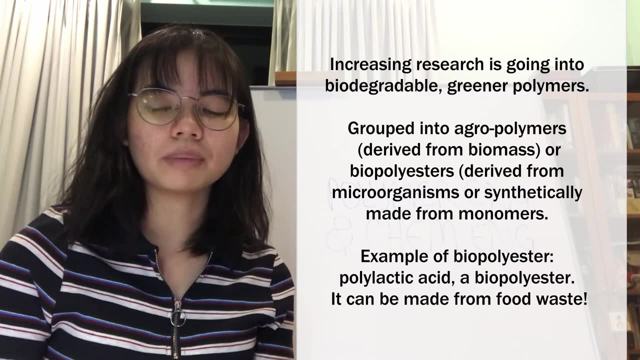 polylactic acid had the second highest consumption volume of any bioplastic in the world, but despite this its use is restricted as it is quite fragile and not compatible with many manufacturing processes. Thus it has to be strengthened with additives. Polylactic acid can be made from food waste, which solves a large environmental and economic. 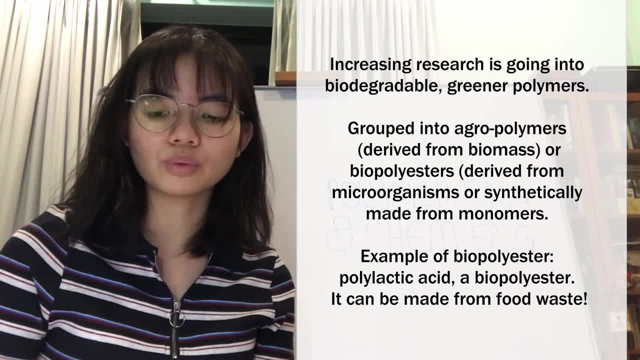 problem, as it means that the anerobic content is low and thus the energy consumption is low. Polylactic acid can be used to produce food waste, which is also a source of food-based. anaerobic decomposition of the food waste will not lead to increased carbon emissions. 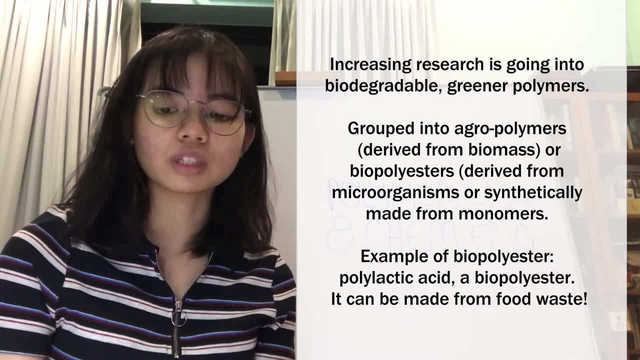 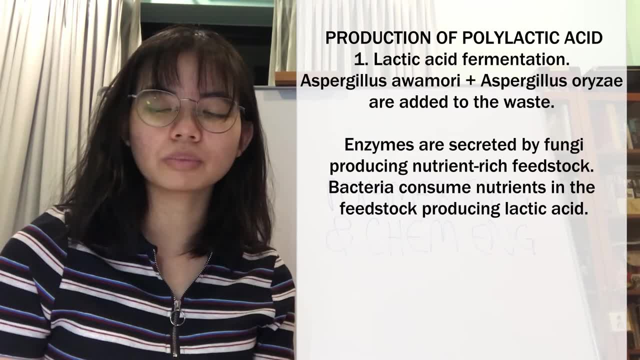 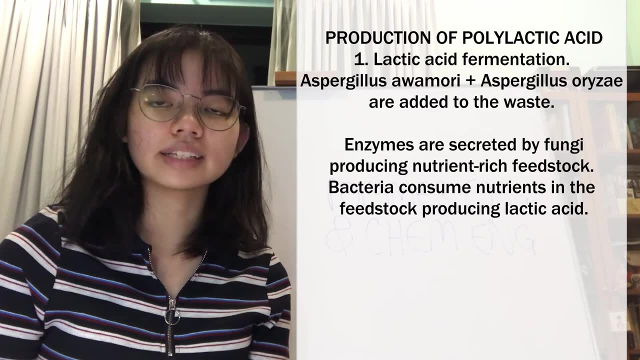 and it means that plastics can be made without additional economic investments into the raw materials for the plastics. Polylactic acid is produced in the following process, created by polymer engineers and chemical engineers, so that it can be mass produced. Firstly, lactic acid is synthesized from fermentation feedstock, from food waste. 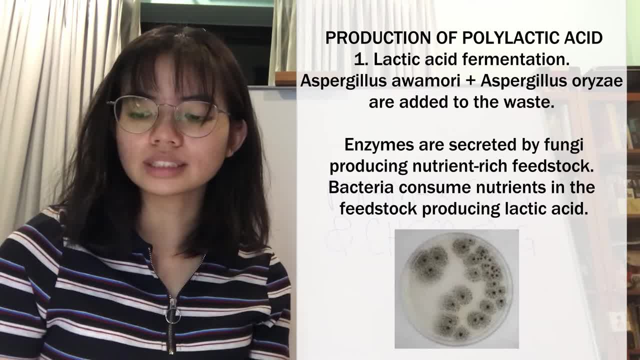 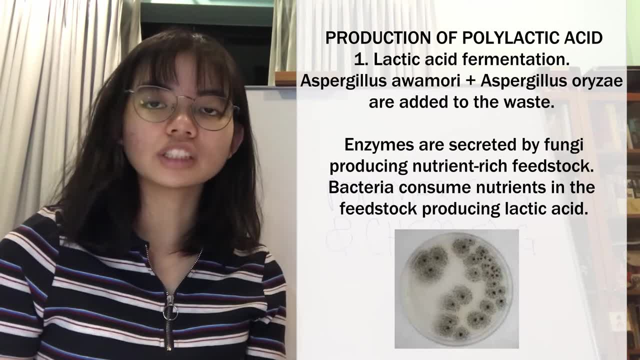 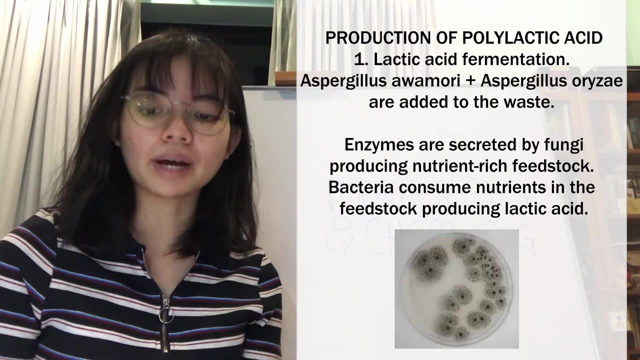 To utilize food waste as fermentation feedstock. Aspergillus awamori fungi and Aspergillus arosae fungi are added to the food waste. Enzymes are secreted by the fungi through solid-state fermentation. The fungal mushes are then blended with the food waste and undergo hydrolysis in a bioreactor. 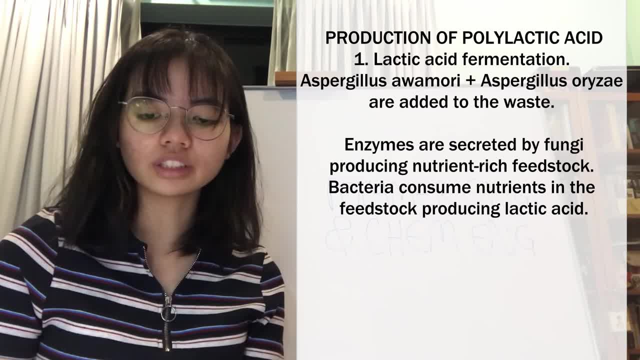 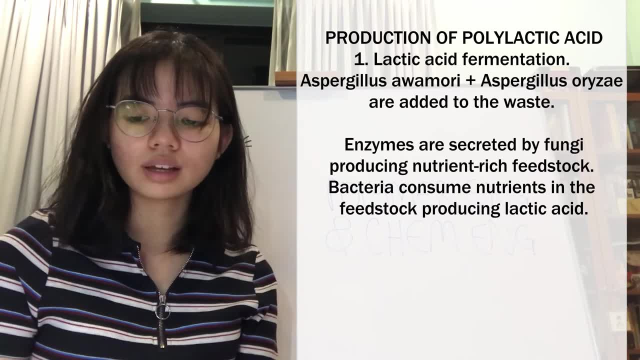 producing a nutrient-rich fermentation feedstock. Bacteria then consume nutrients in the feedstock, producing lactic acid. To recover lactic acid from the feedstock cell, biomass and impurities must be removed by filtration and centrifugation, which is when a mixture is separated through rapid 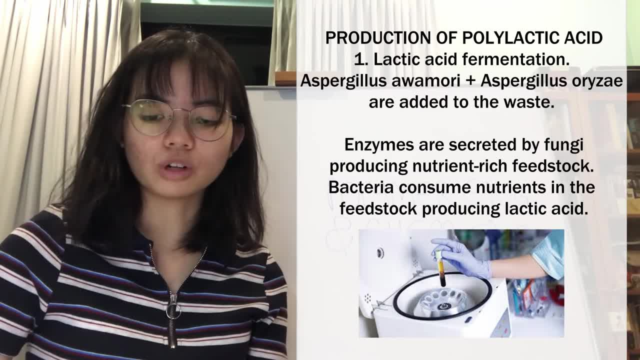 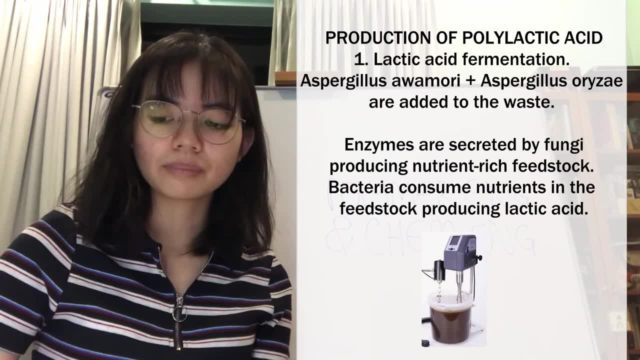 spinning for 30 minutes. Colored impurities are absorbed after mixing with activated carbon, and the solution is then concentrated through evaporation and extracted using ultrasonic methods. The resultant solution is separated with an ethyl acetate solution in a separatory funnel. 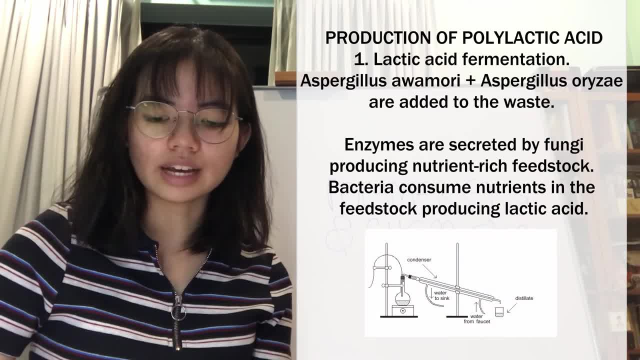 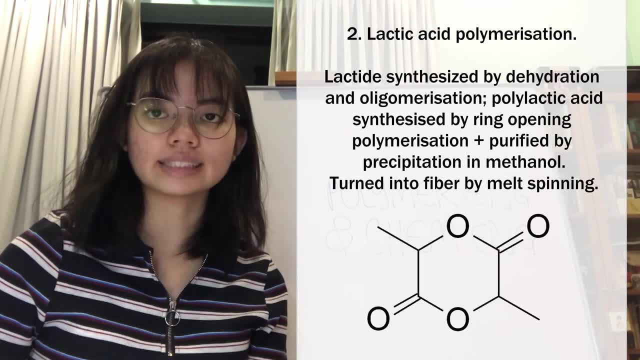 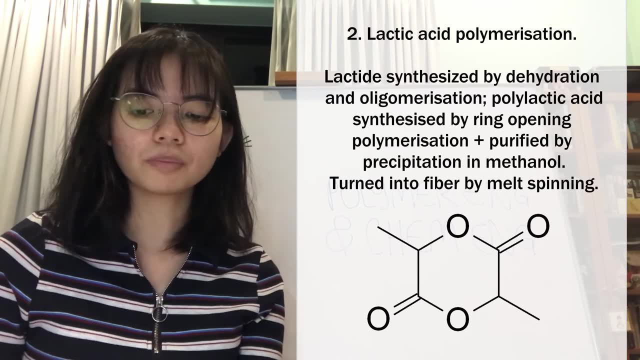 and isolated from the ethyl acetate by distillation at 40°C for 30 minutes. The next step is lactic acid polymerization. Lactic acid is synthesized from lactic acid by dehydration and oligomerization, which is a chemical process that converts monomers into macromolecular complexes or oligomers.